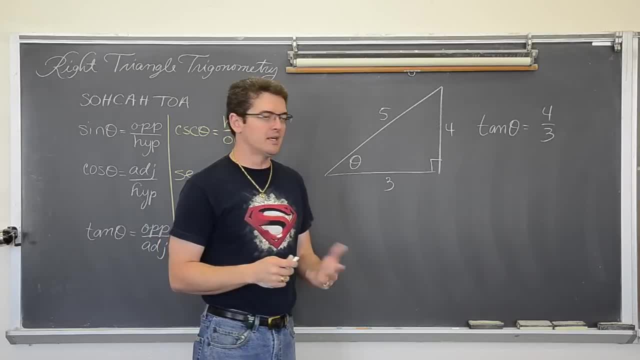 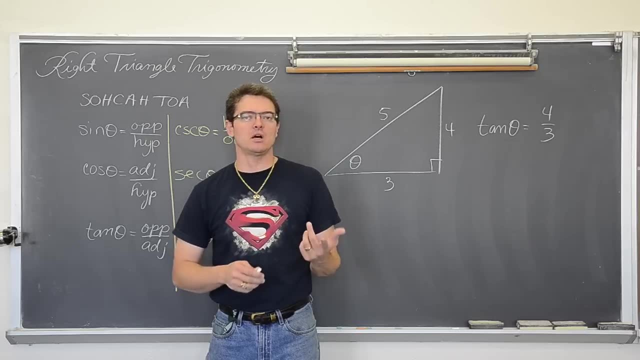 And now we need to get that tangent function away from theta. Well, if I said 2 times x equals 10, you would do the inverse of multiplication, which is divide both sides by 2 and get x equals 5.. If I said you had x squared equals 16, you would do the inverse function of squaring. 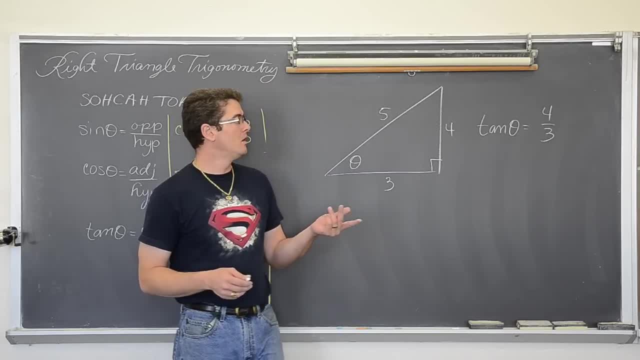 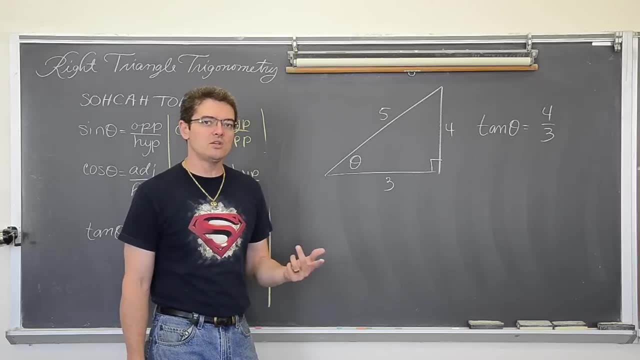 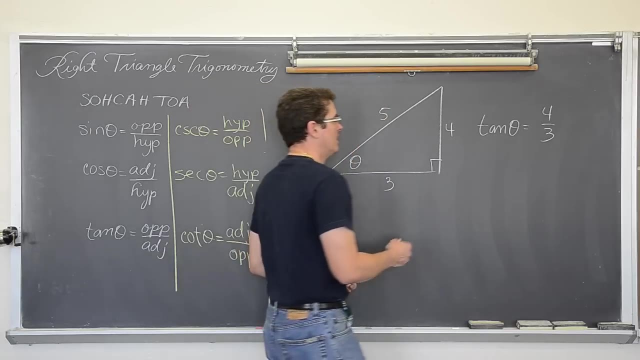 which is square root of both sides, and say x equals 4 and negative 4.. Well, if I want to undo the tangent function, I need to apply the inverse tangent to both sides of the equation. So I am going to write- and this one middle line here may not be necessary for your teacher: 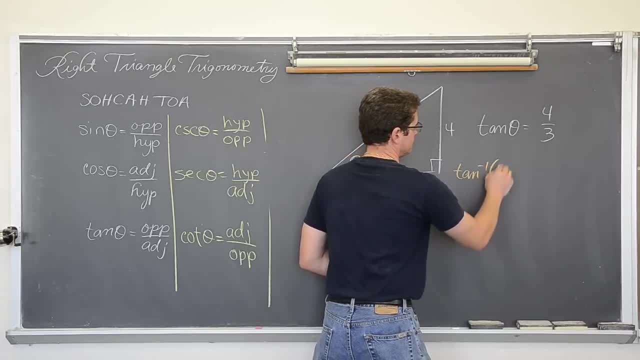 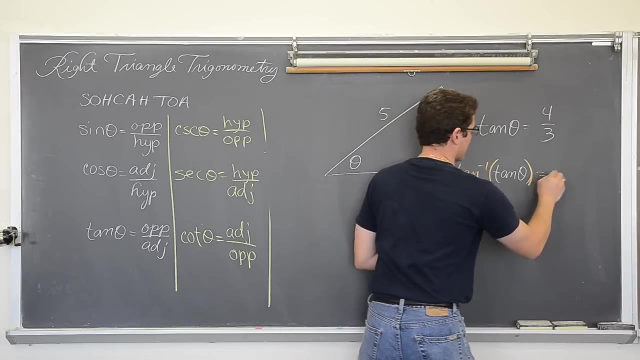 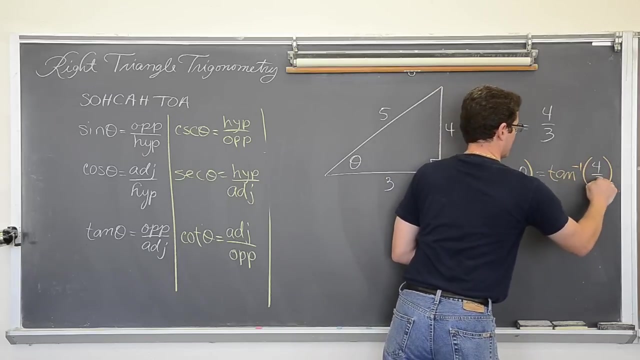 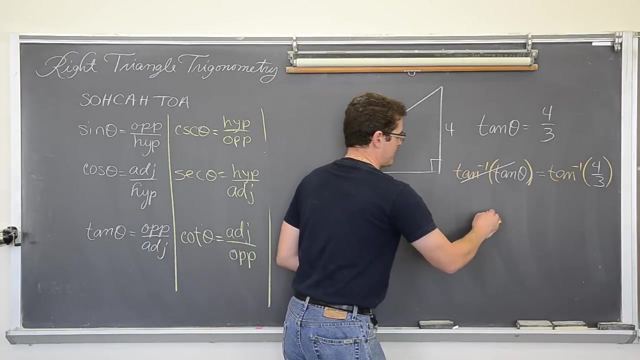 but I am going to apply the inverse tangent- Remember why I am trying to work so hard to color code it. Inverse tangent of 4 thirds and the tangent function and the inverse tangent will cancel each other out, and that is why this is sort of a teaching step. You don't necessarily 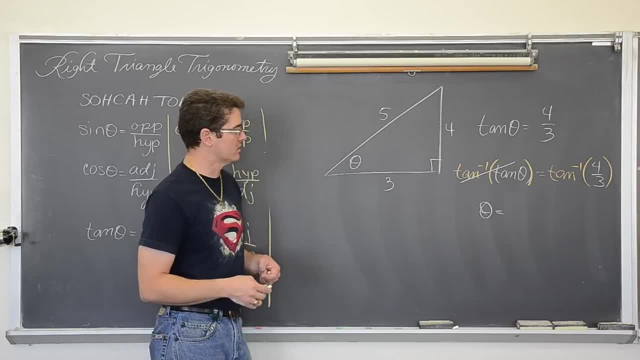 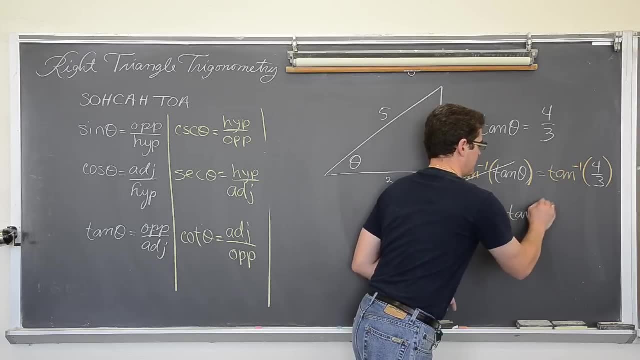 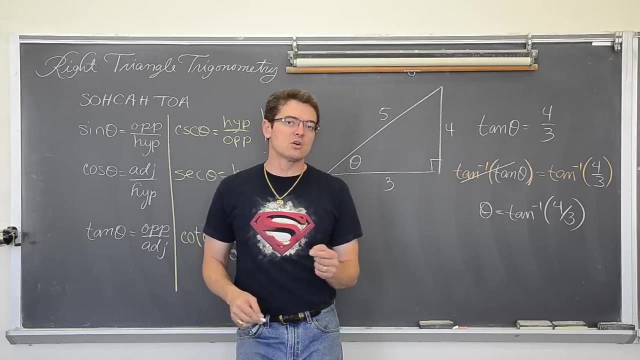 have to show this for just doing triangular, right triangular or whatever you want to do for trigonometry. But theta is going to be the inverse tangent of 4 thirds. Now again, if you want your answers to be in degrees, please make sure that you have your calculator. 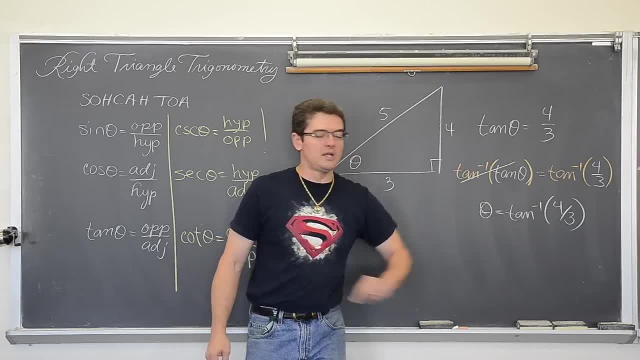 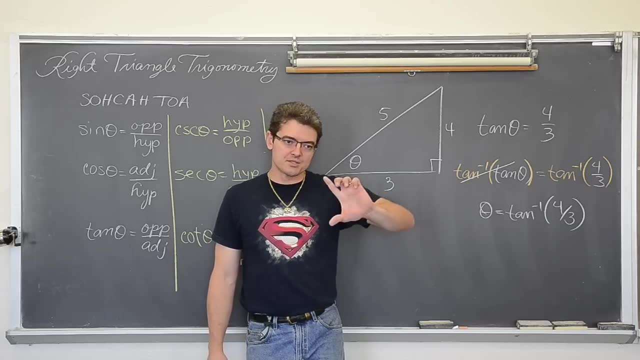 in degree mode And the little negative 1 does stand for an inverse function. Now, 2 to the negative 1 is 1 half 2 thirds to the negative, 1 is 3 over 2.. So a lot of times we 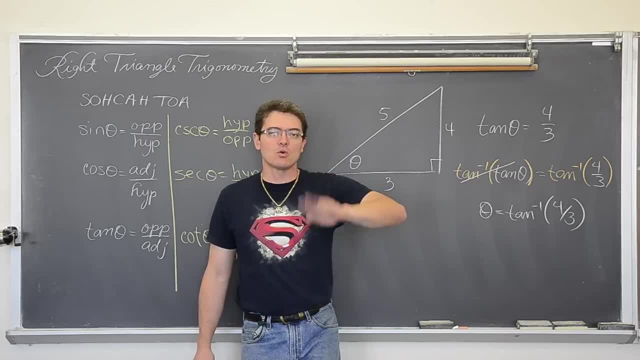 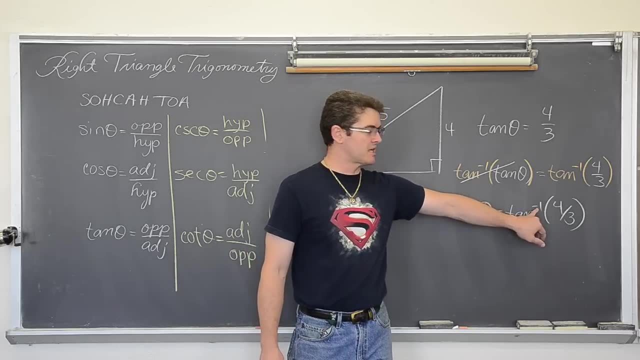 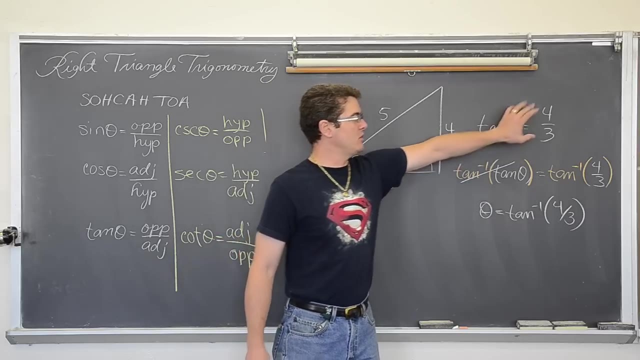 see these negative exponents as just flipping the base or moving the base on which that negative exponent sits on. But when you talk about math functions, this is an inverse math function. What do you put into a trig function, An angle measure, and you get out as we can. 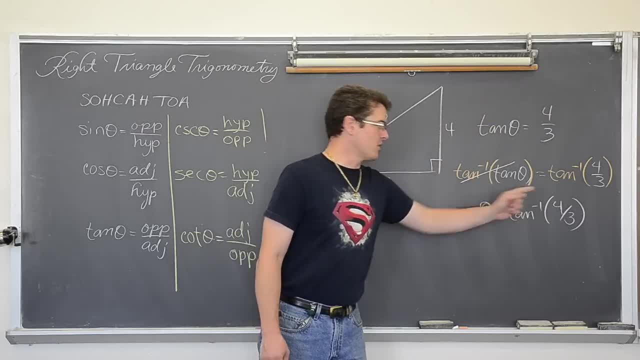 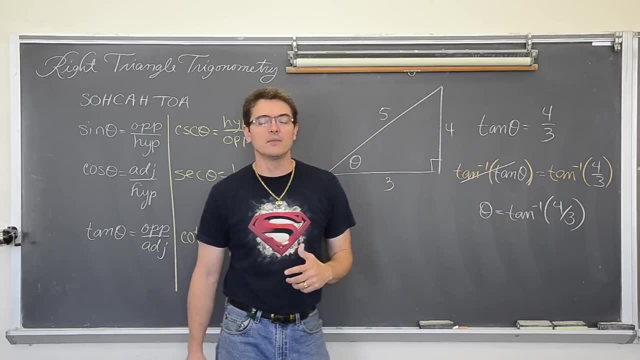 see the sides of a triangle With an inverse trig function you are putting in the sides of the triangle. even if it is just a decimal, like 1 point 3, repeating That is a trig function. That decimal does come from the ratio or the division of two sides of a right triangle.